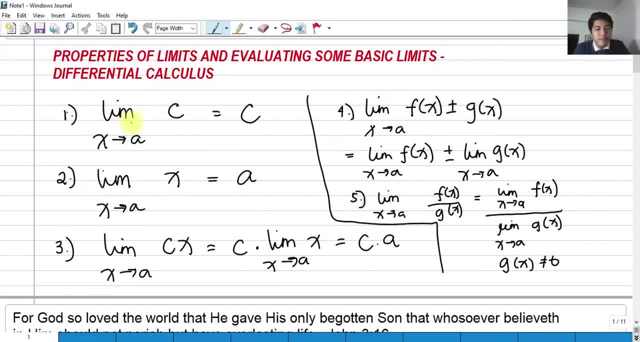 So for number one, we have the limit of C. This is read as the limit of C as X approaches A. Again, this is read as the limit of C as X approaches A is equal to C where C is any constant number. 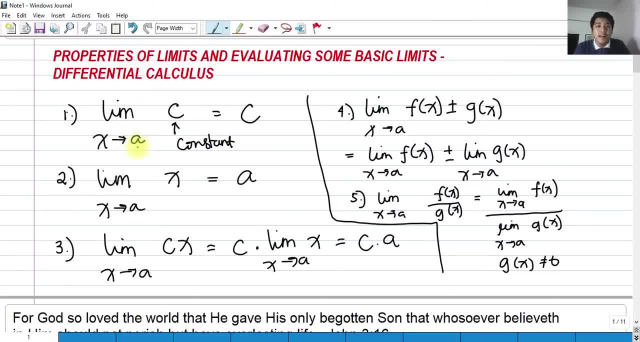 And A is any constant number, A real number, real value. we can substitute. So if we evaluate the limit of a constant as X approaches A, that is only equal to the limit of or to the constant itself. So the limit of a. 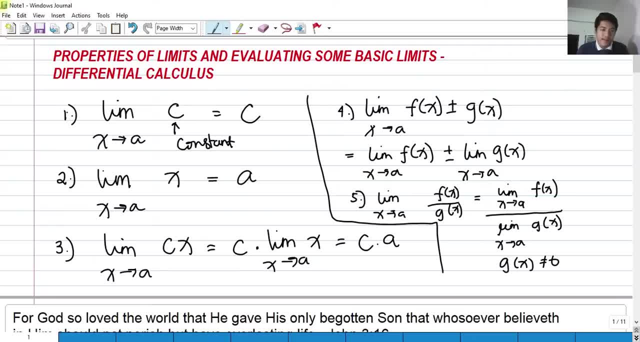 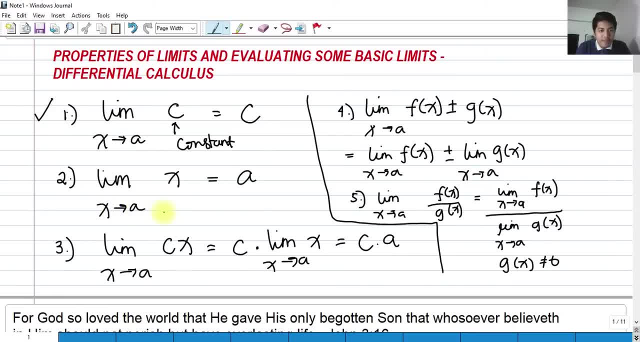 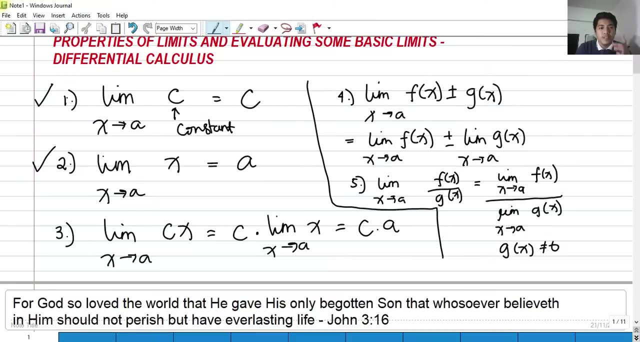 approaches a certain number, real number a, it should be equal only to what is the value of a. okay, so that's property number two: limit of X. as X approaches a is equal to a. so let's, for the first problem, let's, let's have an example, okay. 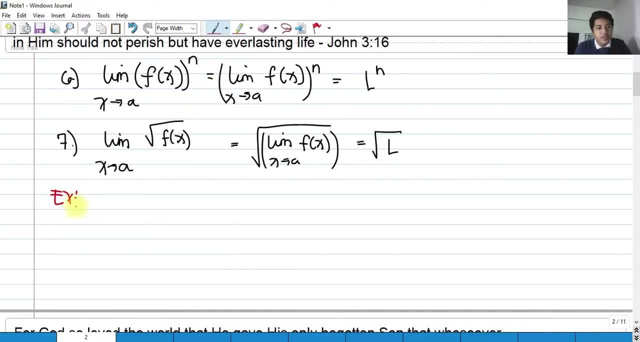 so it says: for our first problem, the limit of a constant as X approaches a is simply equal to the constant. so, for example, if we have to evaluate the limit of two as X approaches one, okay, so this is a constant, this is our C and this is. 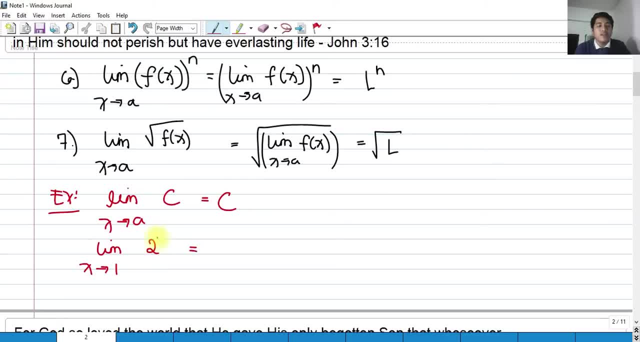 our a. so if we evaluate the limit of a certain constant, okay, as X approaches. a notice that there are no any X term here, so it says by property number one, whenever we evaluate the limit of a constant, that is considered okay, that is equal to the constant itself, which is: 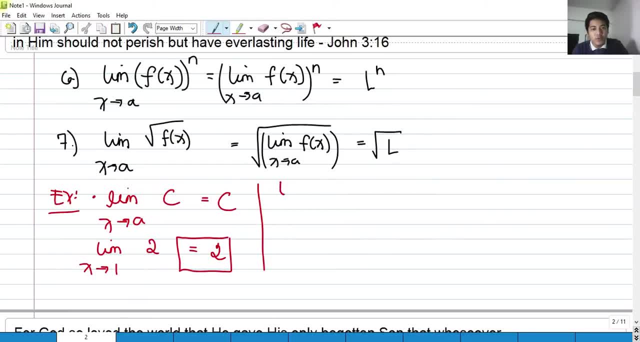 this. that's for number one. how about for number two? the limit of X as X approaches 2 is equal to what. so the property that we have seen a while ago is this: the limit of X as X approaches a is equal to a. so, if we evaluate the, 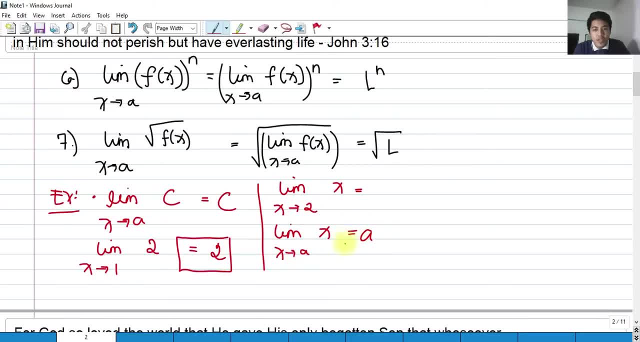 limit of X. as X approaches a, that is only equal to b case, we have an a that is equal to 2. so if we are, if we have a function f of X simply equal to X and evaluate its limit, it should be always equal to the value. 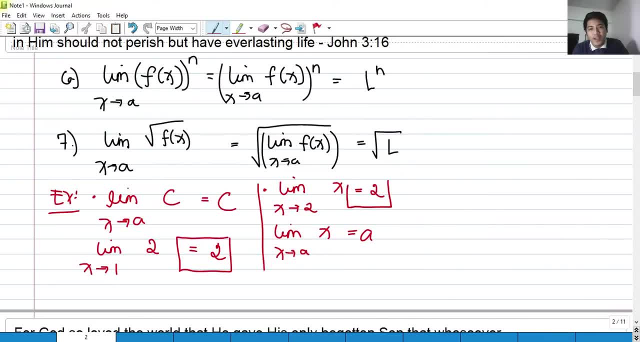 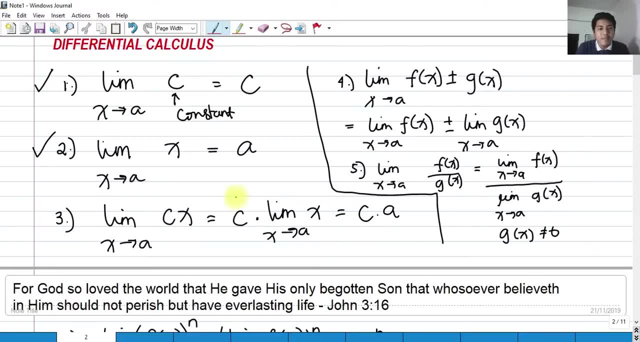 of a, which is, in this case, 2, right. so it's very simple for the first two properties. how about for the third property, the limit of a constant multiplied by X. alright, as X approaches, a is always. we can factor out the constant outside of the limit and multiply it by the remaining f of X. 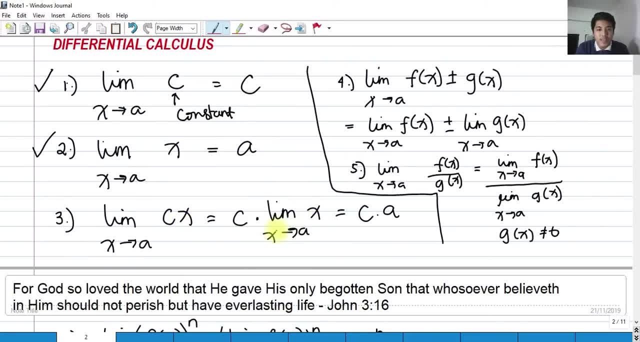 inside. so we have the C multiplied by limit of X as X approaches, a is only equal to, to the constant multiplied by a. since this term is from the property 2, i, this whole thing is equal to the property 2, the limit of X as X. 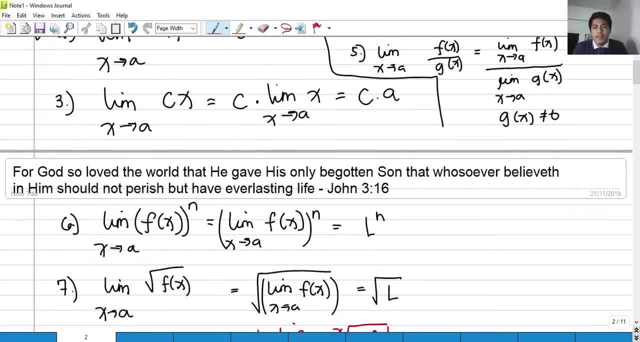 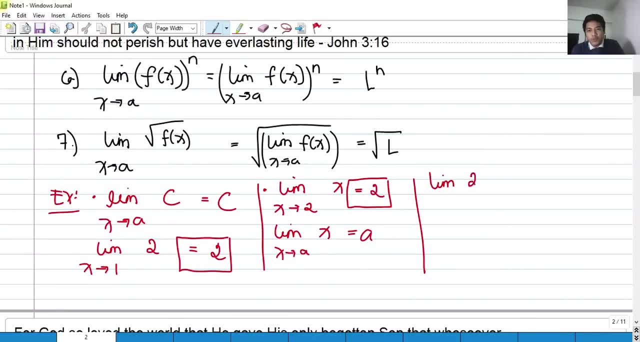 approaches a is 0.5 раз to the unknown, and the value is equal to 0, for the is simply equal to a. so how do we apply that? okay, so, for example, if we evaluate the limit, okay, the limit of 2x as x approaches 2, okay, so what we can do here is to rewrite this. 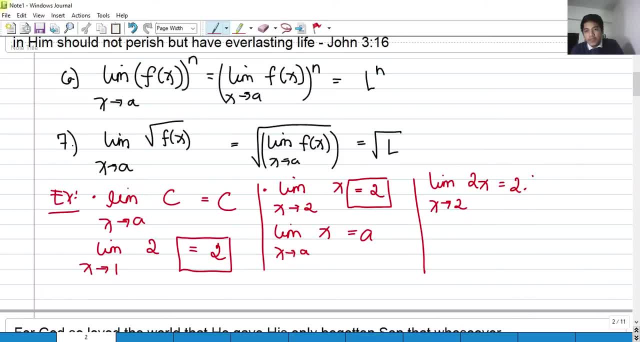 we have a constant 2 here, 2 multiplied by the limit of x. okay, as x approaches 2, and if we evaluate this, okay, this has a similar property to our property number 2 wherein, if we evaluate this, this should be only equal to- that's right- 2. we simply substitute the value of the a here in. 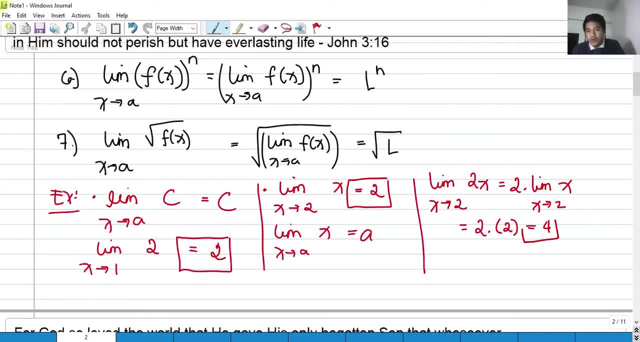 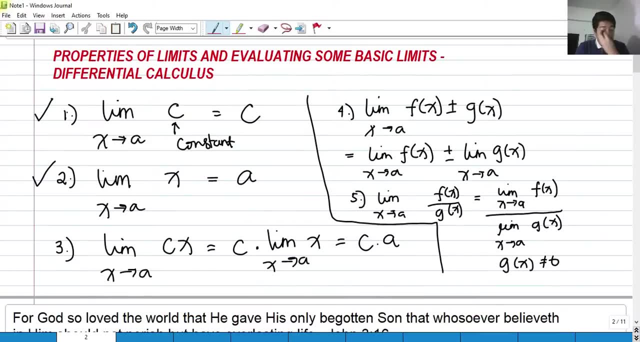 our x. so 2 multiplied by 2 is that is equal to 4. that is what the property meant. okay, means so number 4. this is the limit of two functions: f of x, g of x, in addition and subtraction as x approaches. a notice that we can distribute the limits. 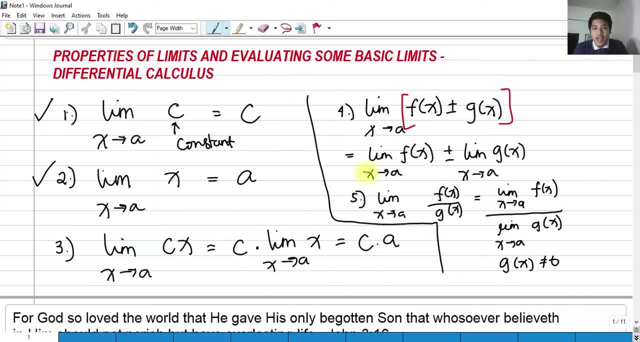 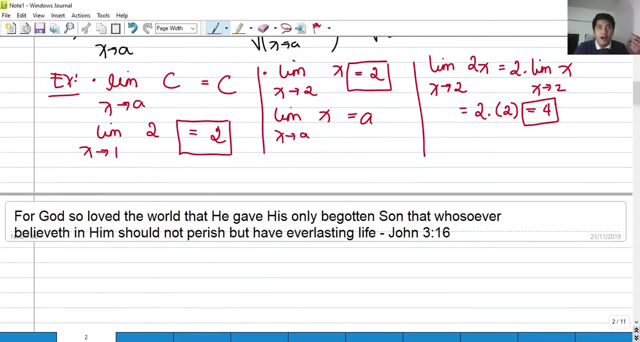 such that we can evaluate first the limit of f of x as x approaches to a plus minus the limit of g of x as x approaches to a. okay, so we can distribute the limits if we have a product or if we have some indifference of the f of x. so let's try to have an example we have. 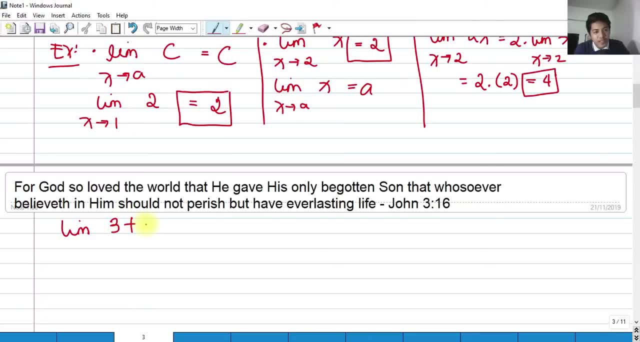 a, the limit of 3 plus x. okay, 3 plus x as x approaches negative: 1. okay, so first, since this is an addition, we can multiply this. okay, but we can actually separate them. so we have the limit of 3 as x approaches negative: 1 plus the limit of x as x approaches negative. 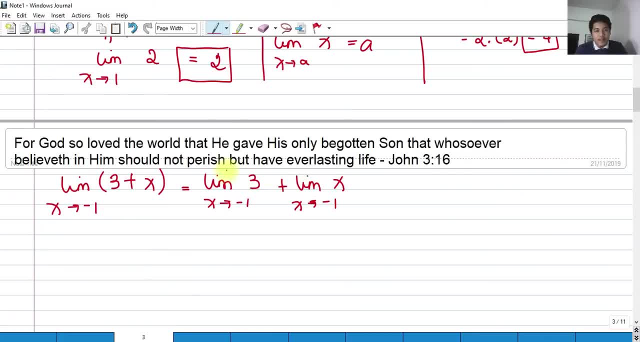 1. so first we can evaluate this left side. so we have the limit of a constant. this is a constant number. as x approaches negative 1, that is still considered as the constant itself. 3, okay, and the limit of x as x approaches negative 1. this is our x, this is our a. if we have again an x, f of x only. 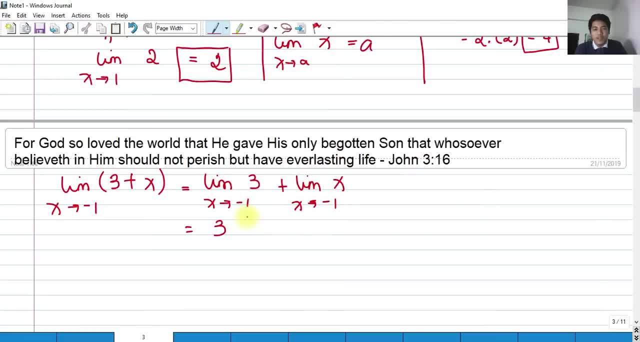 we can simply substitute the value of negative 1, so the limit of this. don't forget the plus. we have the plus here. okay, as x approaches, negative 1 should be negative 1, so that if we evaluate this, this should be 3 minus 1. 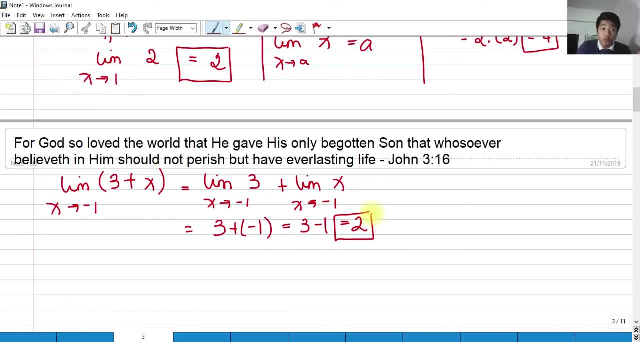 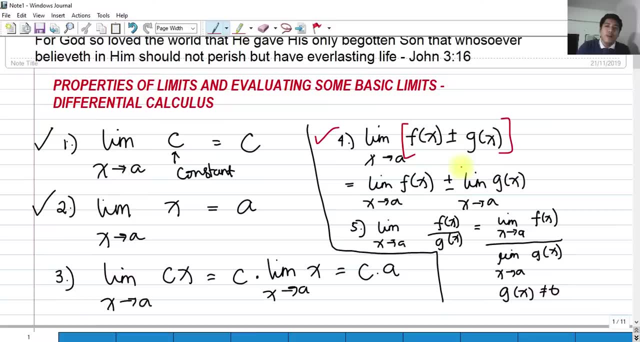 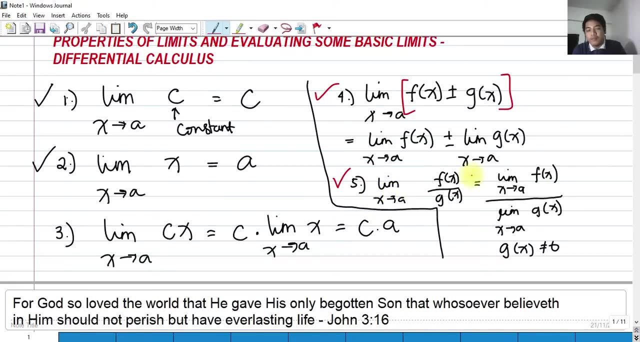 the limit that we are trying to find is equal only to 2. that's what this same for a subtraction, right, we only subtract the two limits. okay, for number 5, the limit of f of x over g of x as x approaches a is the same. we can distribute the limit sign on the numerator such that we have the 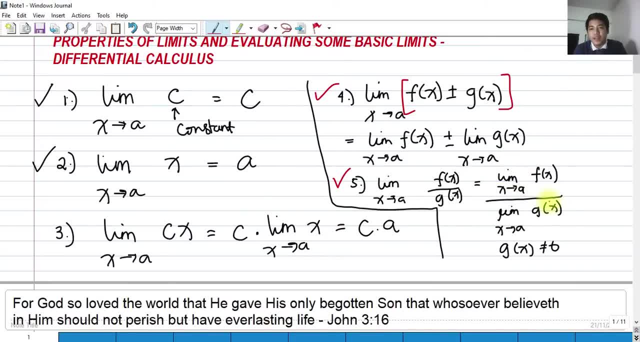 the limit of f of x as x approaches a divided by the limit of g of x as x approaches a, given that the g of x or this denominator should not be equal to zero, because if the denominator becomes zero, okay, we have an undefined function. okay, so we have an undefined. so any number divided by zero. 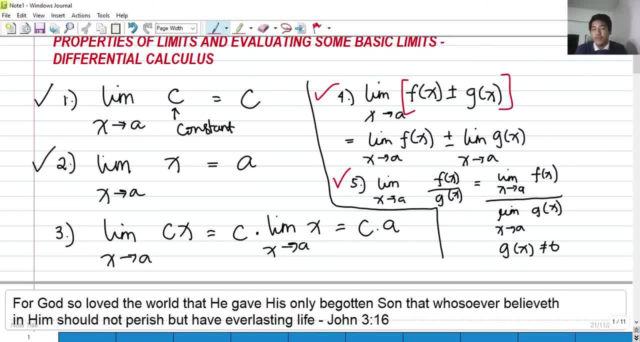 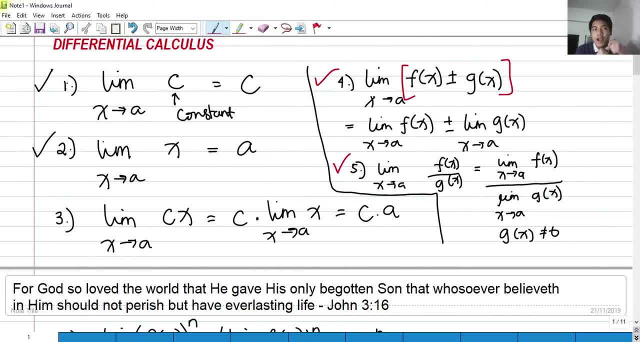 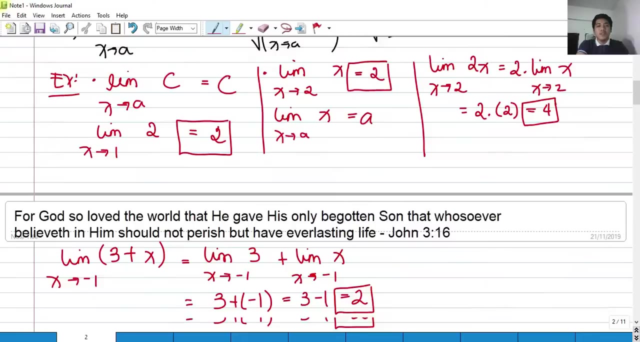 okay, we have an undefined word. of course, if zero over zero, that's indeterminate four. so the rule is: if we are going to evaluate the limit of a uh, let's say uh, we have a uh. what do you call here? a quotient? okay, a quotient. so we must avoid the denominator to get zero. okay, so to demonstrate, 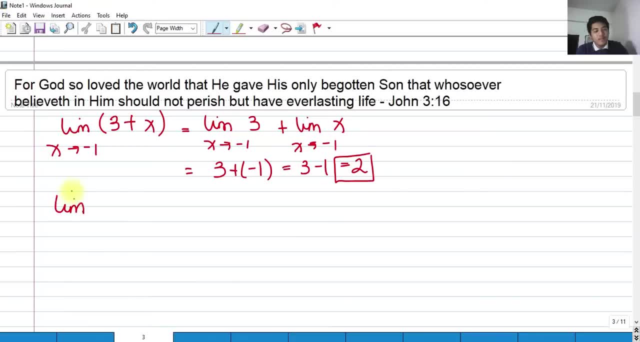 that property. let me show you to evaluate the limit of, let's say, two over x as x approaches four. okay, so we can actually distribute the limit limit of two as x approaches four over the limit of x as x approaches four. okay, from our property, the limit. 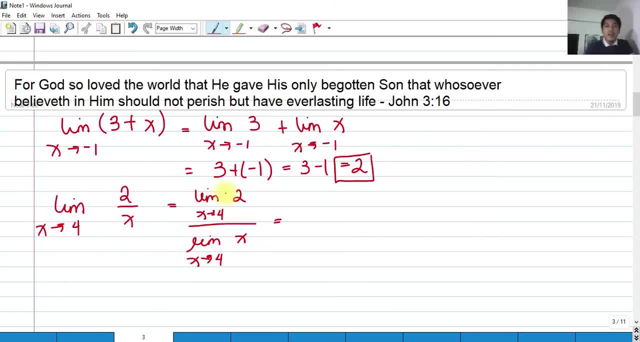 of a constant is a constant itself. the limit of two as x approaches four is simply equal to: yes, that's right. two, because this is a constant, okay, and this the limit of x as x approaches to four. we simply substitute the value of four to the x, so we have two fourths, or in other words, 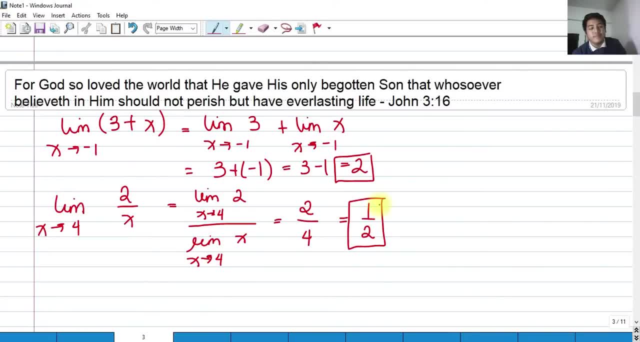 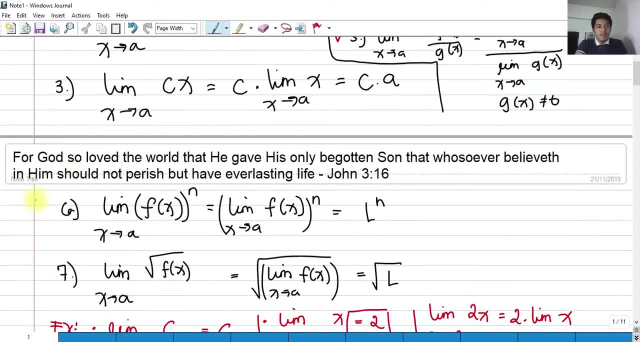 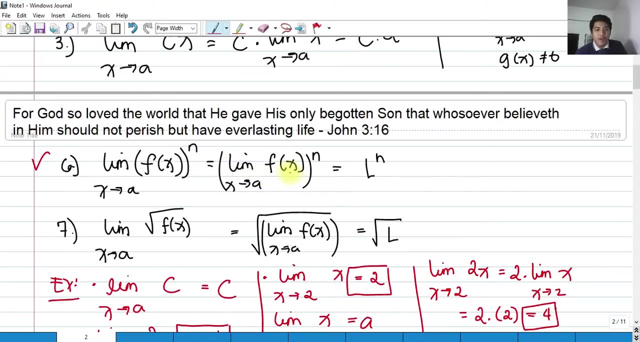 we have one half okay one, so that's we should avoid the denominator getting zero. okay for number six. the limit of f of x raised to n as x approaches to a is simply equal to the quantity limit of f of x as x approaches to a raised to n. or if we have this kind of type of 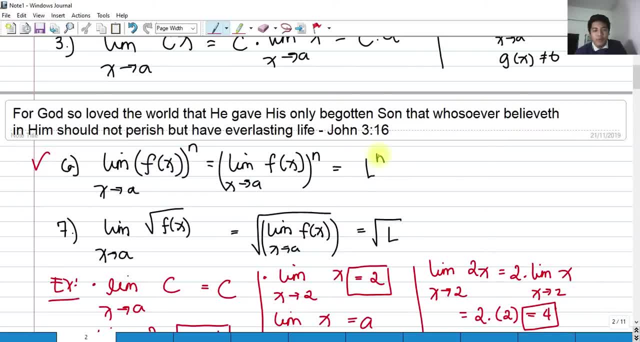 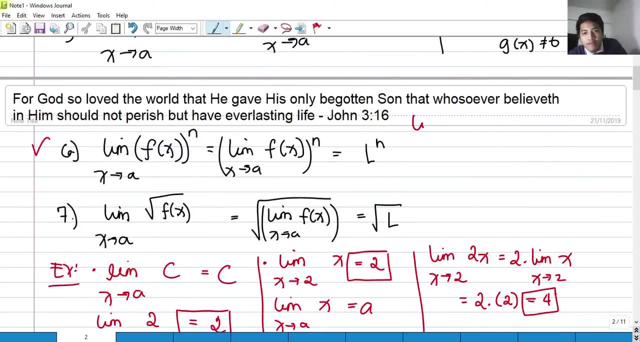 uh, limit, okay, we can evaluate the limit l and we raise it to a certain number and, okay, that is in the exponent. so, for example: so if i, if i want to find the limit of x squared as x approaches two, okay, so i can rewrite this as the limit quantity, the limit of x as x approaches to two. 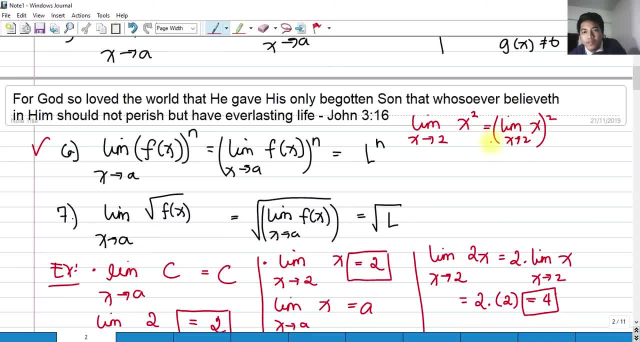 squared. so if i'm going to evaluate the inner part, okay, the inner part, the limit of x. as x approaches two, that is simply equal to two. agree with me, because that's what the property is trying to say. now, don't forget that we have squared here, so we have four, okay. 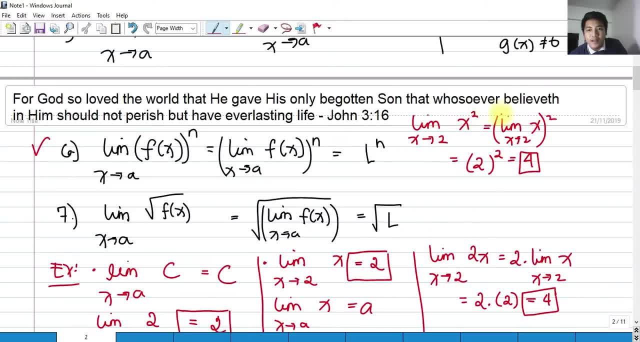 so we can always do that, or we can, uh, actually directly substitute two here in in order for us to evaluate the limit, no problem with that? okay so, but still, i'm going to show you the properties. so, lastly, for our uh number seven. we're going to show you the properties. so, lastly, for our number seven. 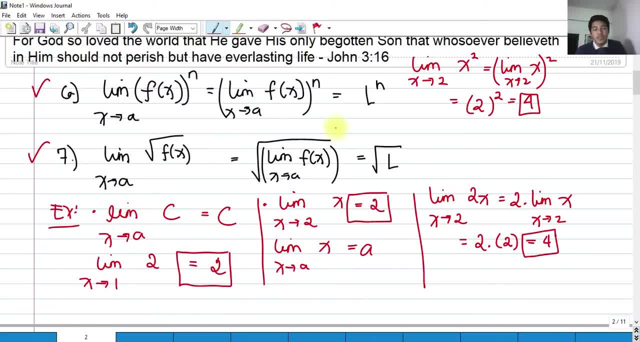 property. the limit of the square root of m of x is, as x approaches to a, is simply equal to the square root. the quantity of the limit of f of x, as x approaches to a is simply equal to the square root of l, where l is the the result of the limit. so let's try the limit of square root of 2x as x. 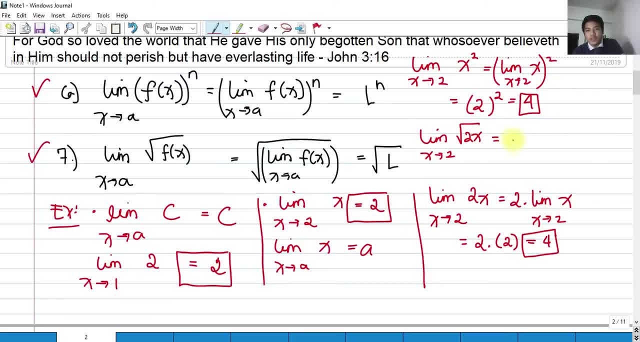 approaches two is we can actually what have this? the limit of 2x? okay, x approaches two. so we can evaluate the limit of this. okay, the inside. so we know that if we simply substitute two here, we will be having we can factor out, i mean, we can factor out two limit. 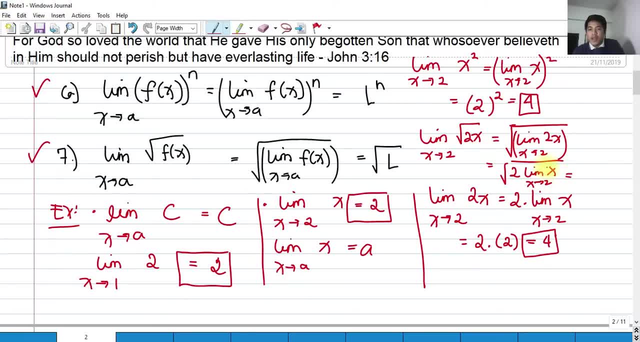 of x as x approaches two. so we have now, as x approaches two, that is square root of two. limit of x as x approaches two is two times two. now square root of four would become simply equal to two. all right, or we can simply substitute the value of a, all right, here inside. 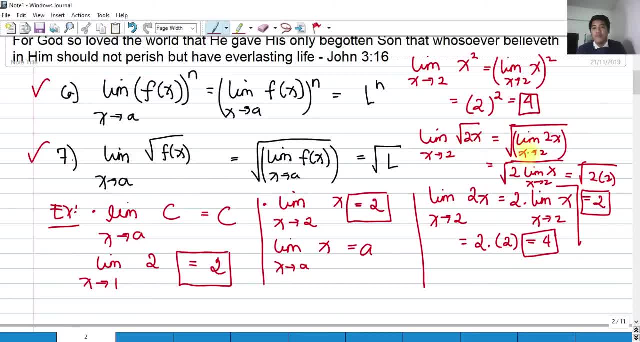 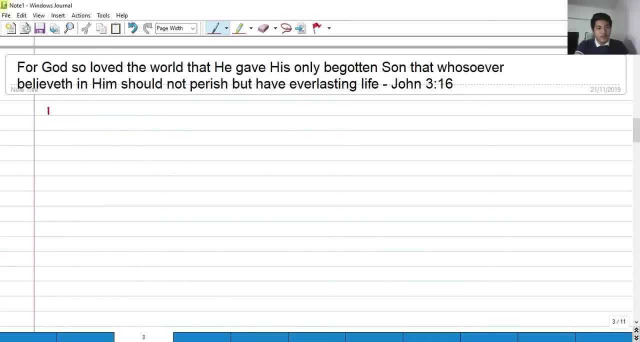 the radical sign all right in our x and evaluate the limit, okay. so now let's try to solve some problems, okay, involving limits. furthermore, okay, so we have the limit. find the limit of x squared minus four x as x approaches two. okay, so we have here a polynomial. 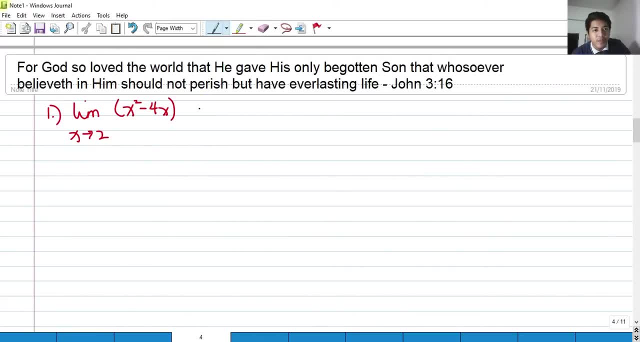 so how do we evaluate the limit of this? using the properties of our limits? okay, by sum or and product or sum and difference. so we have limit of x squared as x approaches to two, minus the limit of four x as x approaches to two. okay, so using the properties, we can have right this limit, the limit of x. 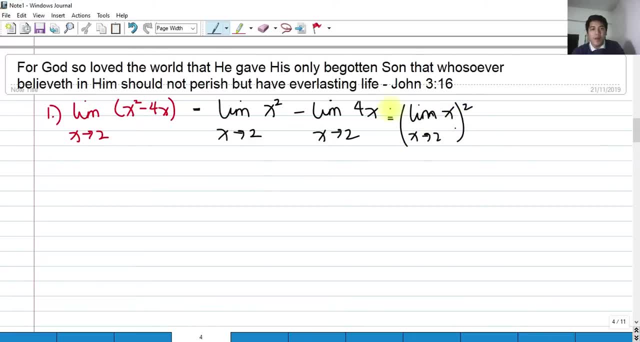 as x approaches two squared. okay, applying the property minus, i can factor out four outside of the limit because it's a constant. so the limit of x now would become x as x approaches to two. so if we evaluate this, the limit of x as x approaches to two, the inside of the quantity. 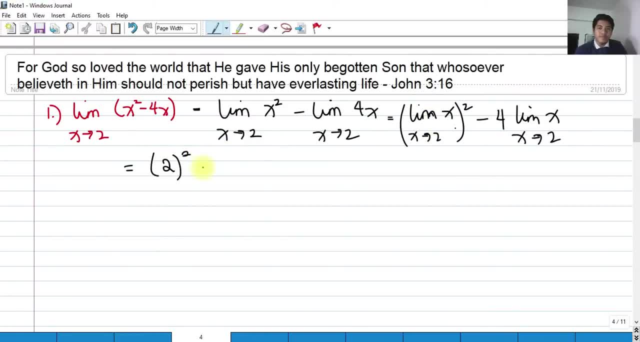 would become two because of the property. so we have two squared minus four multiplied by what is the limit of x? as x approaches two, why is the yesterday gets applied to x? forces of x to x will be x. but alright, again it's x kx. 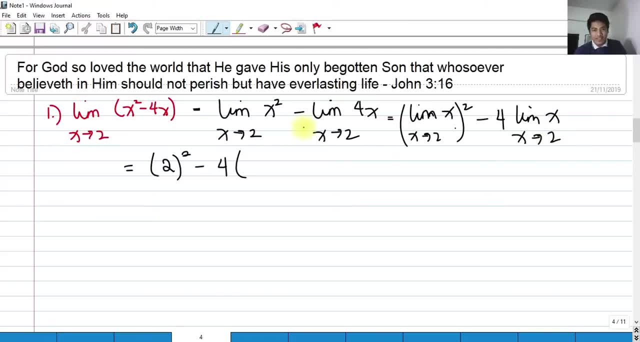 approaches to 2.. Simply we substitute the value of 2 on the x by property, So we have 2.. So that is 4 minus 4 times 2 is 8. And that results to a negative 4.. So another way to solve this. 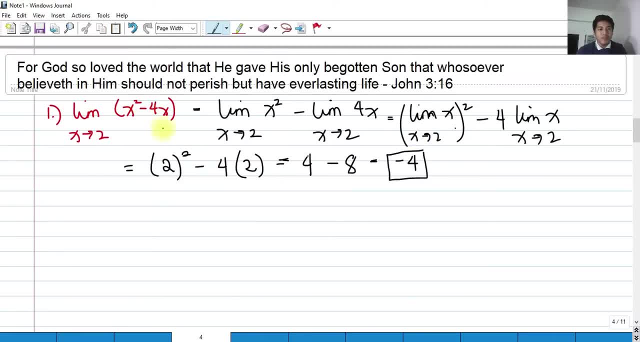 since this is a polynomial function. this is a polynomial in our function. we can substitute directly the value of the x okay, of the value of this a on our x function or our x third. So we can have: 2 squared minus 4 times 2 is equal to 4 minus 8. And that is equivalent to negative 4.. 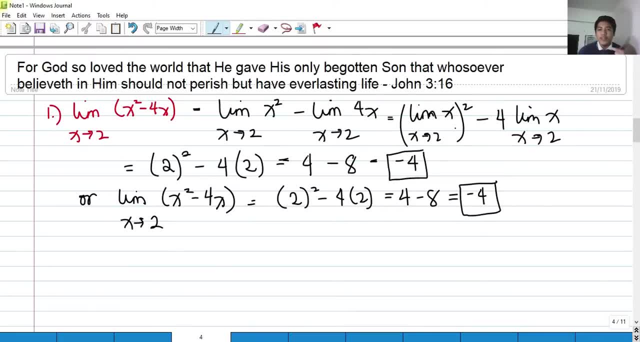 Okay. So if we have a polynomial evaluating the limit of a certain polynomial, we can simply substitute the value of this a to our x's here. Okay, And that's the answer. So for number 2, let's try to solve again another problem. So the limit. 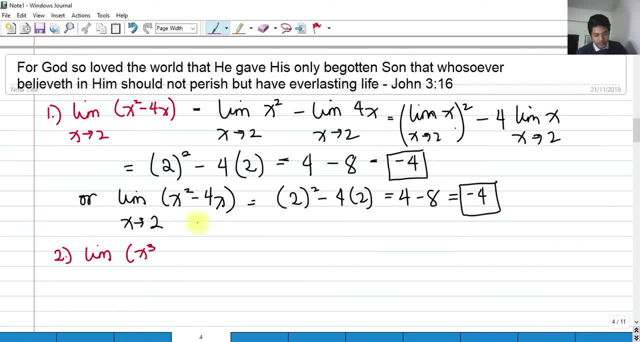 of, let's say, x cubed plus 2x squared, minus 3x minus 4, as x approaches 1.. So, as what I have said a while ago, this is a polynomial, So we can simply substitute the value of 1, okay. 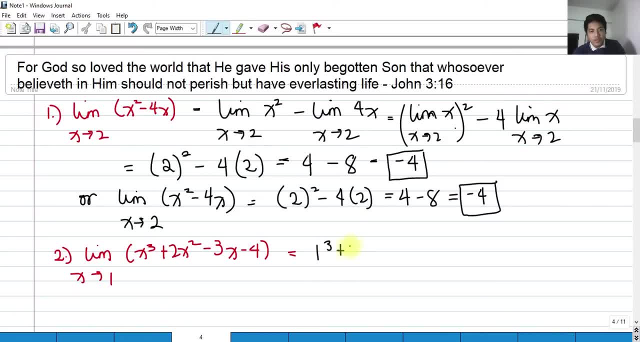 in our x's here. So we have 1 cubed plus 2, 1 squared minus 3 times 1 minus 4.. So we have 1 plus 2 minus 3 minus 4.. Okay, So our answer again is negative 4.. So if you do this addition in 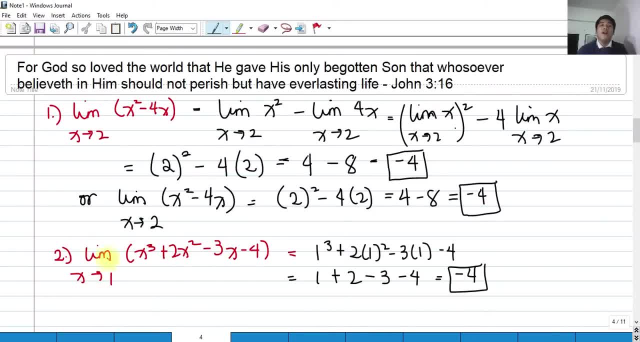 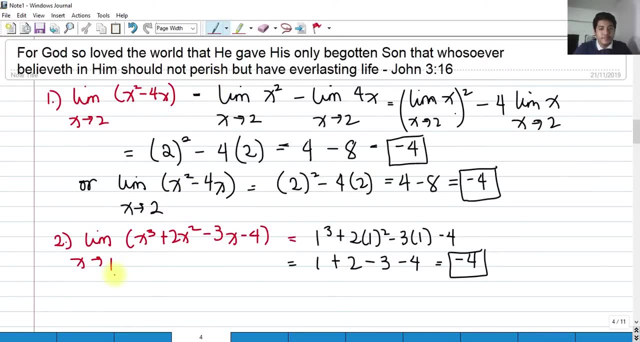 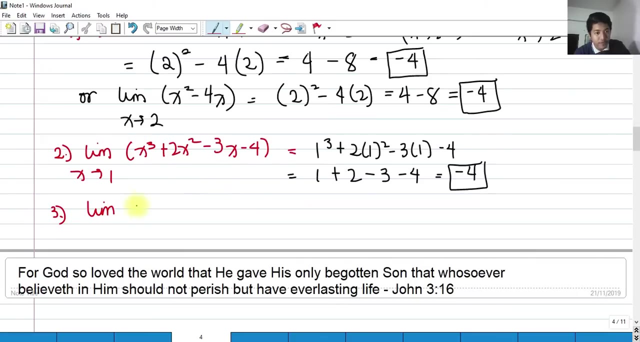 subtraction properties, such that you distribute the limit on n on every, each term, on each term, you will still get the same answer. All right, So let's try again for number 3.. So for number 3, we have to evaluate the limit of 3x minus 1. 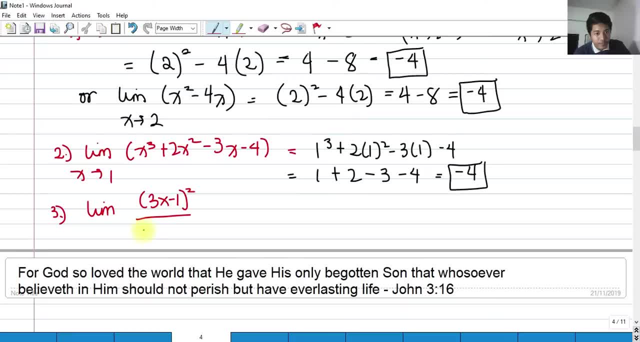 squared over x plus 3, cubed as x approaches 2.. 1. So what is our rule if we are evaluating a cubespace, Not what I am saying? Ah, yeah, Then I will explain how it works again, So that I am because the squareth of 1 at the elétron's gång. So instead, let's try again. So for Number 3, we have to evaluate the limit of 3x minus 1 squared over x plus 3 cubed as x approaches 1.. So what is our rule if we are evaluating a coinspace? 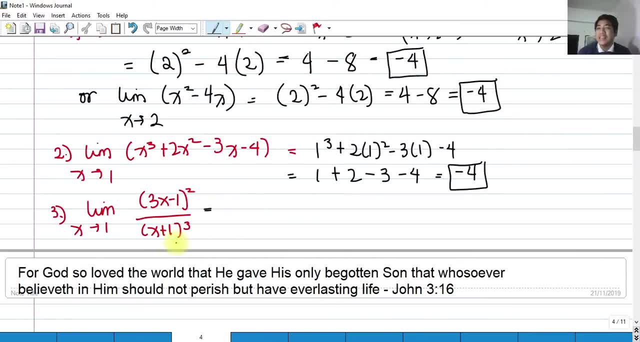 quotient f of x, the denominator should not equal to zero. okay, so what we can do by our property, we can have the limit of 3x minus 1 squared as x approaches to 1, over the limit of x plus 1, cube as x approaches to 1. okay, so, furthermore, we can have this, as we can simply substitute the value. 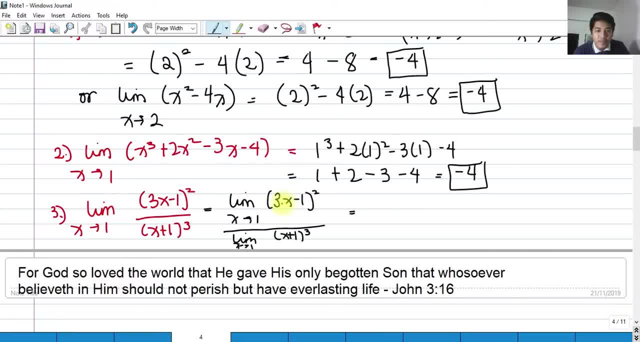 of 1. okay, that is still the same if we try to include or rewrite this square outside of the parenthesis. so we have, we simply substitute the value of 1 for shortcuts. so we have 3 times 1 minus 1 squared. okay, and the same for our values here. okay, for 1. so we have, we can simply substitute. 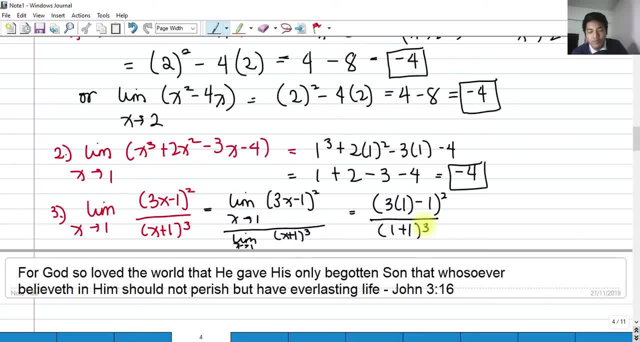 so we have have 1 plus 1 cube, since this is a polynomial. okay. so we have: 3 minus 1 is 2. squared, that is 4 over 2 cube, which is 8. 1 plus 1 is 2, 2 raised to 3 is 8. so that is 1 half in its lowest term. 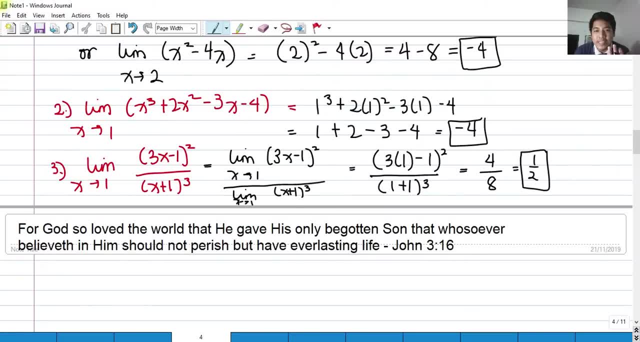 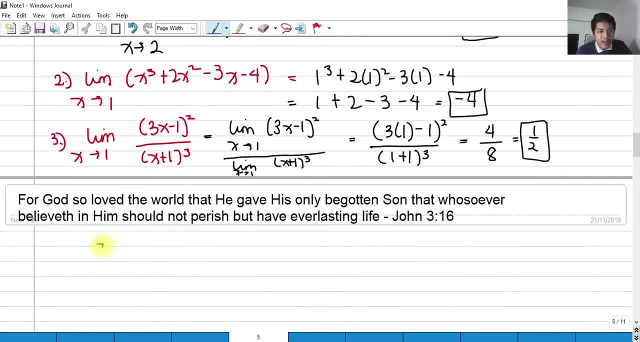 so, again, i didn't show you the whole process of properties, okay, because if we evaluate it, that is still the same. okay, so if you don't believe me, let's try again. so we have the limit, as x approaches to 1, of 3x minus 1. okay, oops, we should not have a parenthesis here. so that is equivalent. 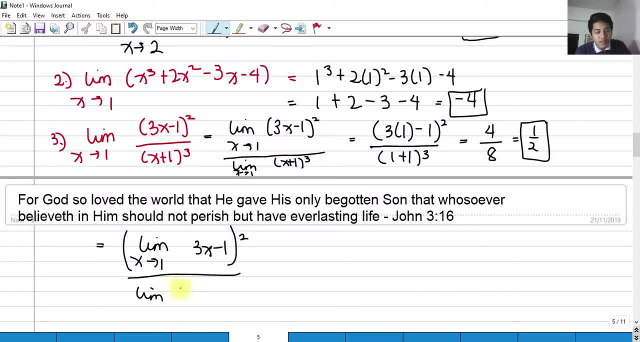 to squared over the limit of x plus 1. okay, as x approaches to 1 of cube. okay, that is still the same. evaluate this. so we have the limit of 3x as x approaches to 1. okay, let me just rewrite the limit of 3x as x. 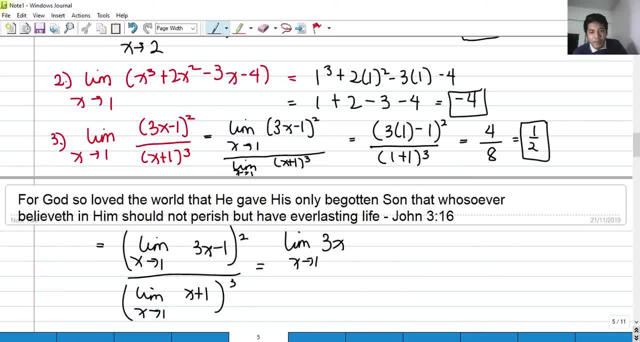 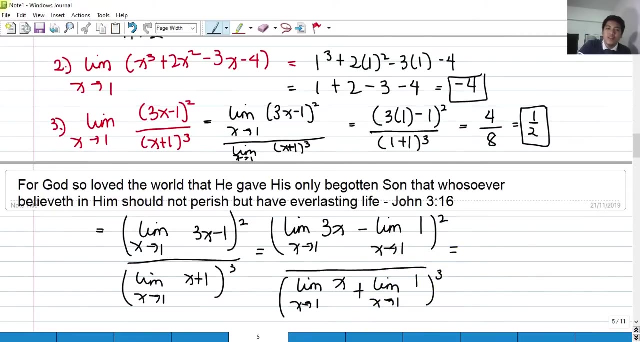 approaches to 1. that is a difference. so we have, minus the limit of 1 as x approaches to 1, squared okay over the limit of x as x approaches to 1, plus the limit of 1 as x approaches to 1 cube. so if you evaluate this, 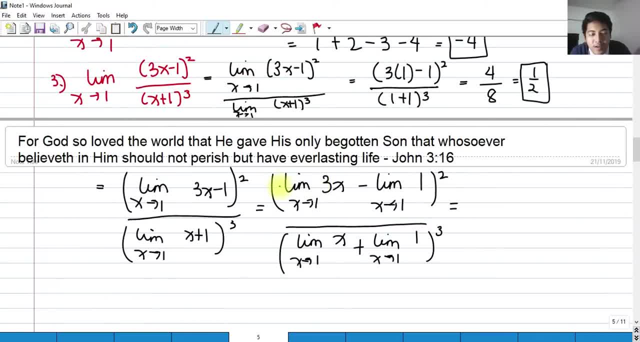 we can factor out 3 outside of the limit- okay, so that i can rewrite this 3 outside of the limit and multiply by the limit of x as x approaches to 1, so that it would become 3 times 1. okay, because the limit of x as x approaches to 1 is 1. okay, minus the limit of 1 as x approaches to 1. and then 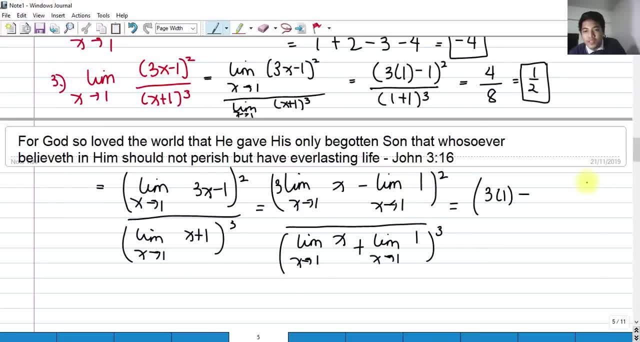 x approaches to one, the limit of a constant one is the constant itself, which is, uh, one. okay, and take note, this is in square, and we have: the limit of x as x approaches to one is simply one by property again, and the limit of one as x approaches to one, one plus one. okay, because this is a 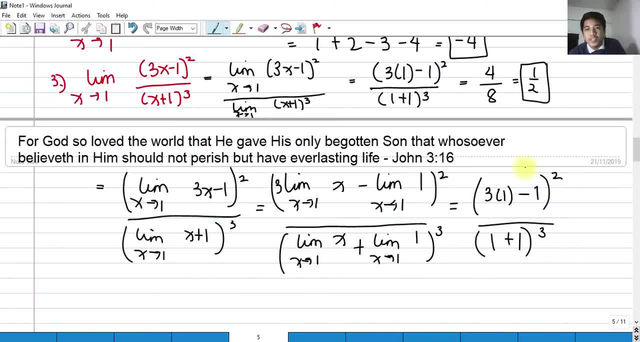 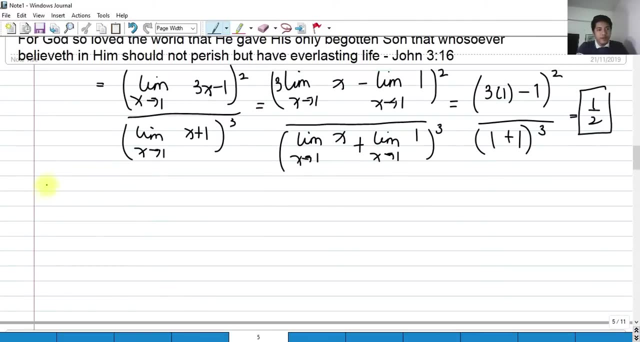 constant. so, and the limit of a constant is the constant itself. so, as you can see, we have arrived at the same uh solution here to here, so our answer in this is still one half okay. so for next problem we have number four: the limit of three raised to x minus three raised to negative. 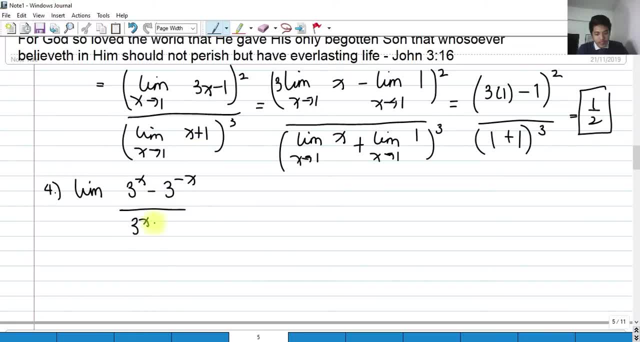 x over three raised to x plus three raised to negative x as x approaches to zero, zero, zero, I. so let me just rewrite this. I don't want to have any exponent that is a negative, so let's simplify that first limit of three x minus. I can bring this down. 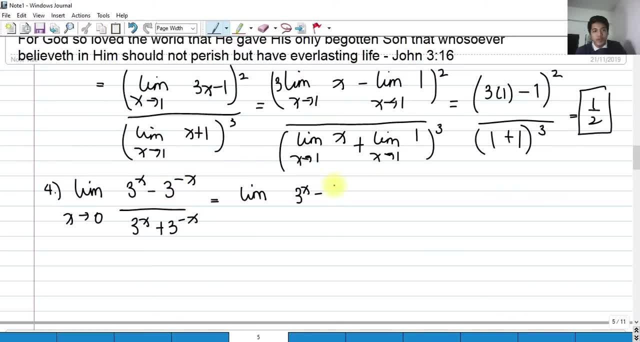 by actually negating and getting the reciprocal of this. so we have, uh, one over three x. okay, that's by properties of exponent. as x approaches to zero, we have three raised to x minus uh, plus one over three raised to x. okay. and if we evaluate the limit of that, the limit of this is by quotient and 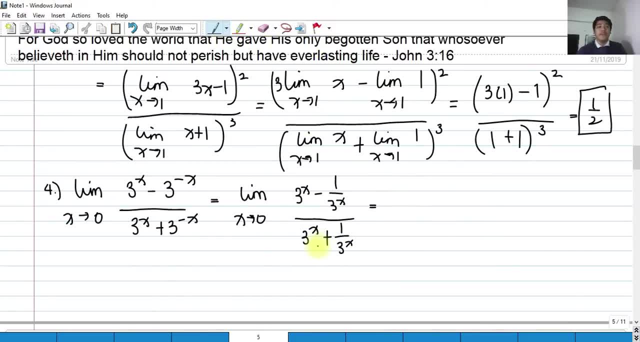 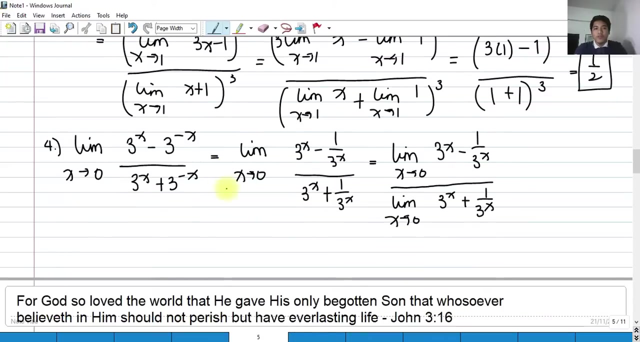 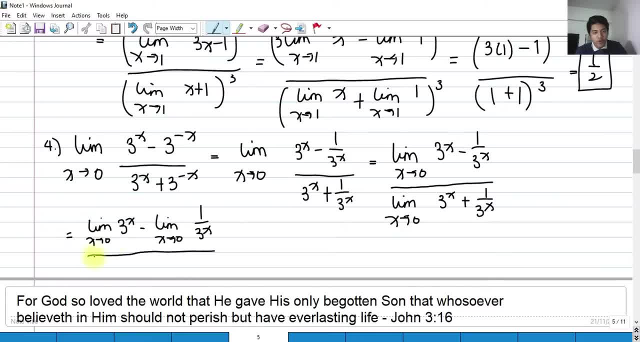 x approaches zero as x approaches zero over the limit of three. raised to x. as x approaches zero, plus the limit of one over three. raise to x as x approaches to zero. okay, so we can simply substitute the values of access here. so we have three raise to zero. okay, the values of a i mean to our x. so we have three raised to zero. 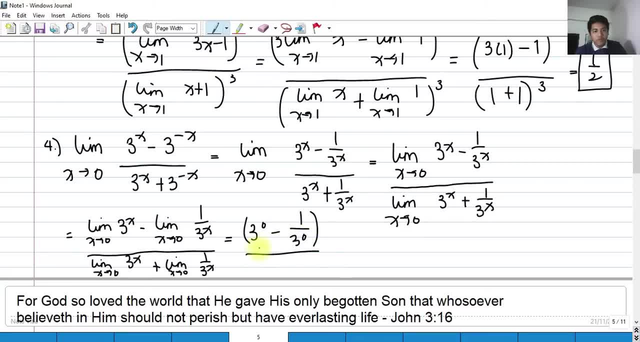 minus 1 over 3 raised to 0 over 3 raised to 0, plus 1 over 3 raised to 0, and any number raised to 0 will be equal to 1. 1 minus 1 over 1. okay, because 3 over 0, 3 raised to 0 is 1. 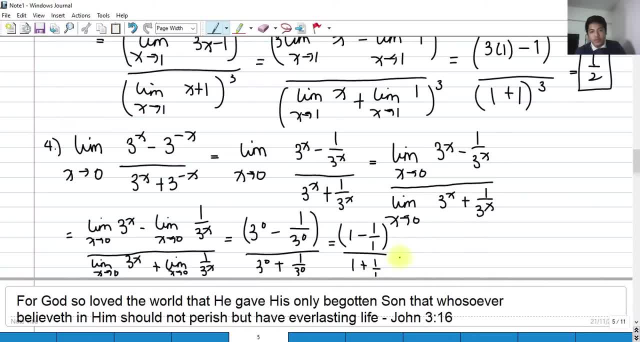 okay, and 1 plus 1 over 1. so we have 1 minus 1 over 1 plus 1, which is 0 over 2. so notice that we have a zero denominator or zero numerator. that's okay, we are trying to avoid, only for the 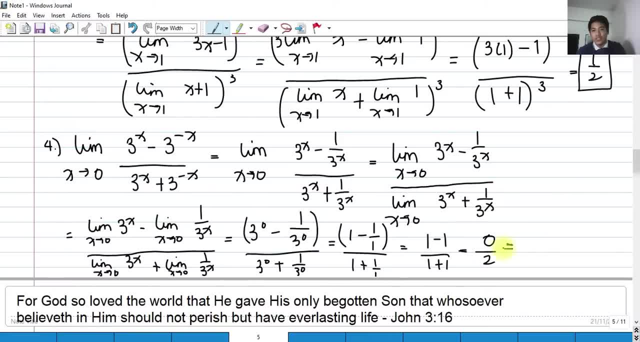 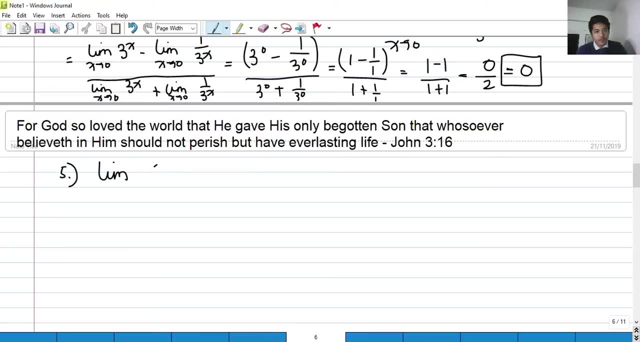 denominator to get 0. so 0 divided by 2, 0 divided by any number would be equal to 0. so that's the limit for this problem. okay, and for number 5. okay, for number 5 we can have the limit of x minus 1 over x squared minus 1. okay. 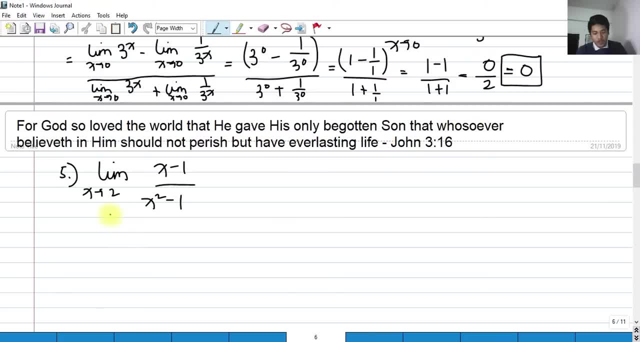 as x approaches to 2. okay, so the only problem here is again, we should not get a zero denominator here upon evaluating the limit. so we can distribute the limit limit of x minus 1 as x approaches 2 divided by the limit of x squared minus 1 as x approaches 2, and by: 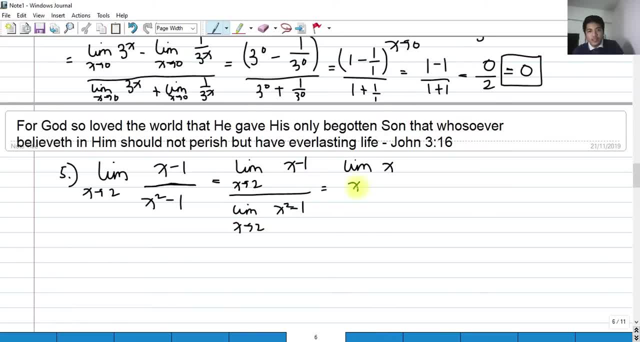 properties. we can furthermore rewrite this as: the limit of x as x approaches 2, minus the limit of 1 as x approaches 2. over the limit, okay of x squared as x approaches 2- okay, minus the limit of x or of 1: okay of 1 as x approaches 2. so 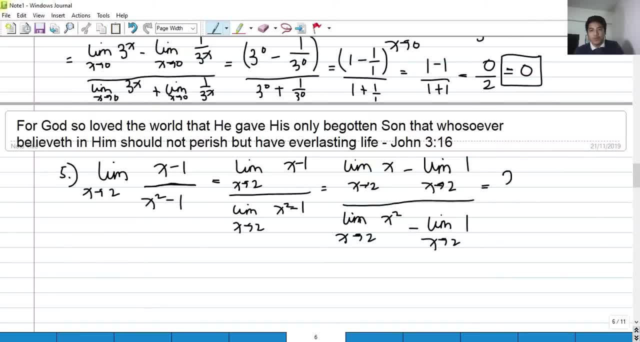 again. the limit of x as x approaches 2 is simply equal to 2. the limit of 1 as x approaches to 2. this is a constant. so what so? the limit of a constant is always the constant itself. okay, which is this? we have the limit of 2 as the limit of x squared as x approaches to 2. that is simply 2. 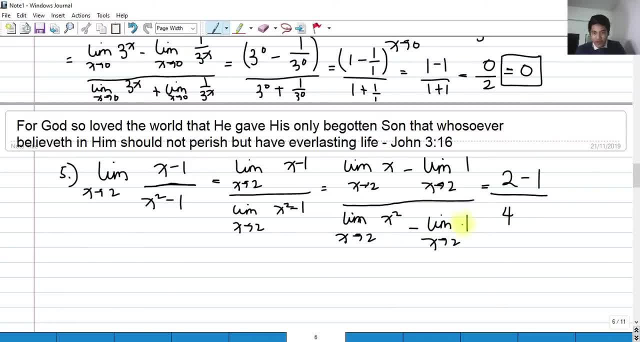 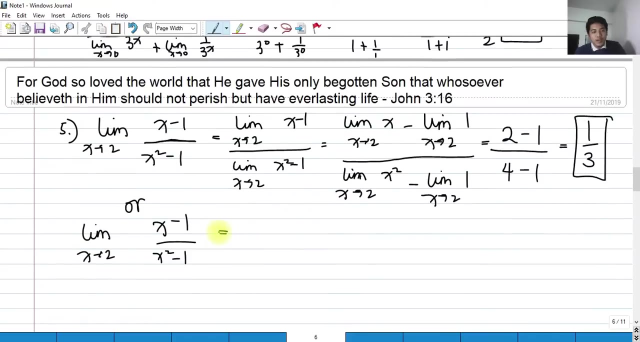 squared, which is 4 minus the limit of a constant as x approaches 2 is simply the constant itself. so we have 1- 3rd. okay, so that is our answer, or from our given, we can simply first simplify the f of x before we evaluate the limit. okay, as you can see here, limit limit as x as limit of x minus 1 over. 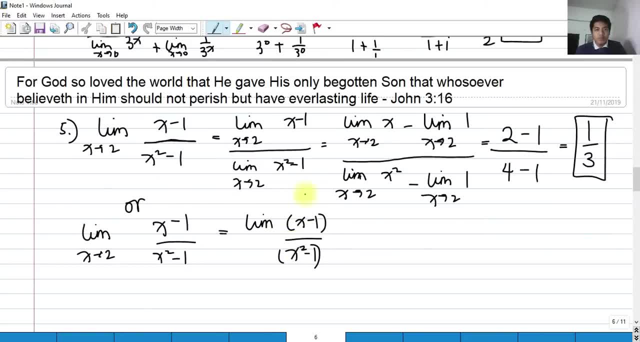 x squared minus 1. okay, x squared minus 1 can be rewritten as x plus 1. okay, x plus 1 multiplied by x minus 1, now it's as x approaches to 2, so we can see here that x minus 1 will cancel. so we have now the limit of 1 over x plus 1 as x approaches to 2. 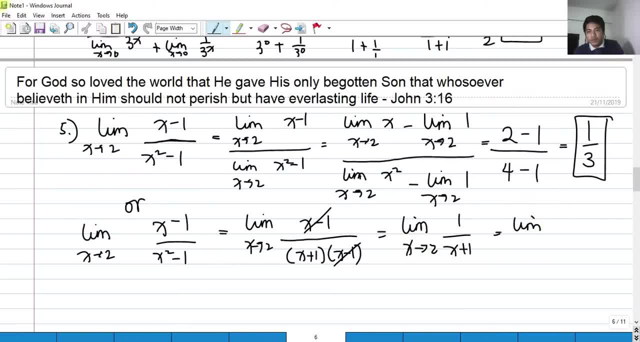 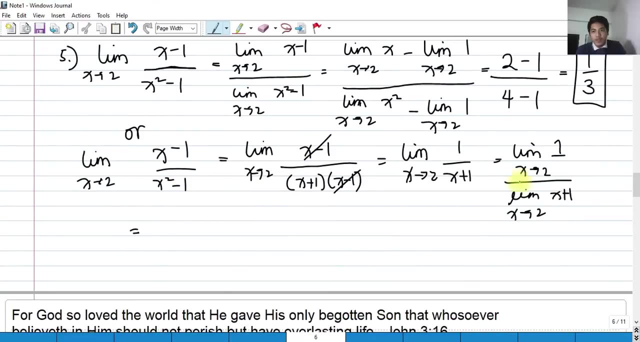 and we can simply what have the limit of 1 as x approaches to 2 over the limit of x plus 1 as x approaches to 2? as you can see here, if we evaluate that that is the limit of 1 as x approaches to 2, the limit of a constant is the constant itself. so we have the limit of x as x approaches. 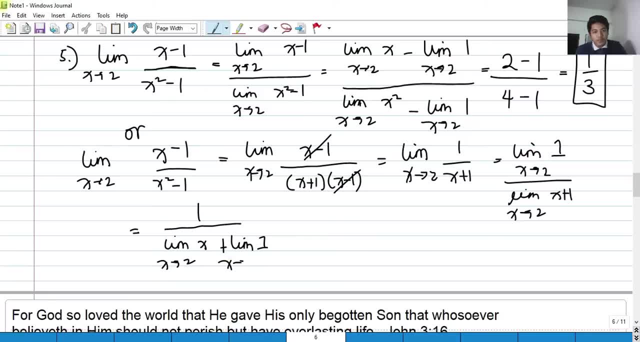 to 2, plus the limit of a constant, 1 as x approaches to 2. so we have 1 over this, the limit of x as x approaches to 2 by property 2, that is equal to 2, the limit of a constant. okay, as x approaches 2. 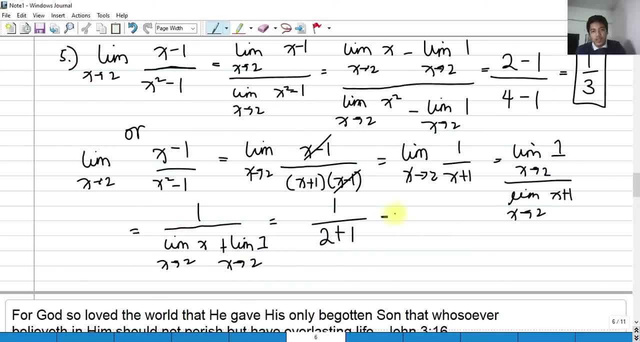 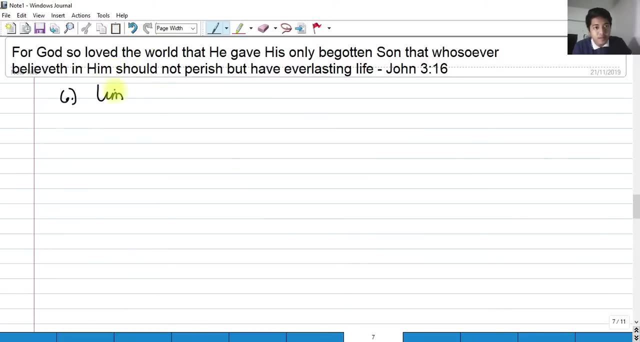 is simply the constant itself, which is 1, so we can have the same answer. okay, so I hope that's clear with you. so for our next problem, for number 6, we can solve number 6, the limit of x squared minus 4 over x squared minus 5x plus 6. okay, as x approaches positive 2, okay, so. 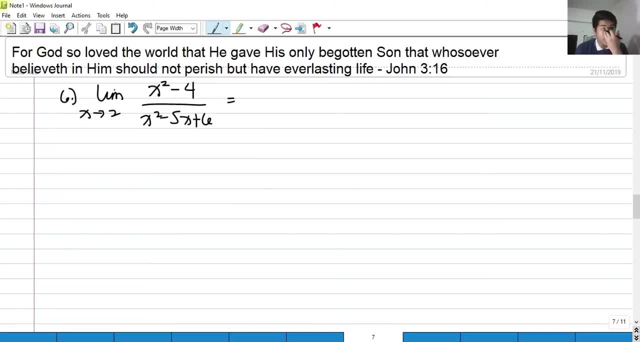 we can. uh, it's easier to evaluate the limit. okay, and since this is a quotient, we are, we are actually avoiding for the denominator to get zero. okay, so for us to have an easier limit, so we can factor out this two polynomial f of x and g of x here on the denominator. so so for us to have 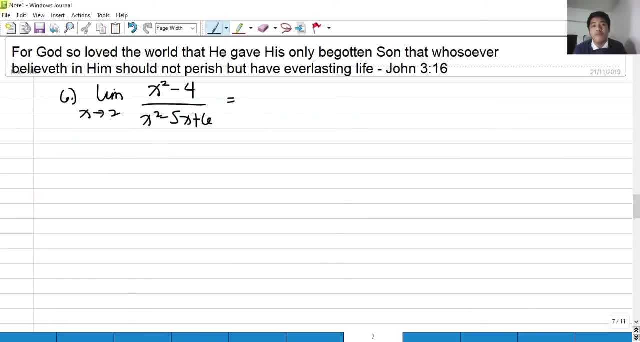 an f of x or function. that is much simpler. therefore, if the function is much simpler, then we can evaluate it for the denominator. so for us to have an f of x or function, that is much easier. so we have the limit. x squared minus 4 is equals to x plus 2, x minus 2. over okay, over x. 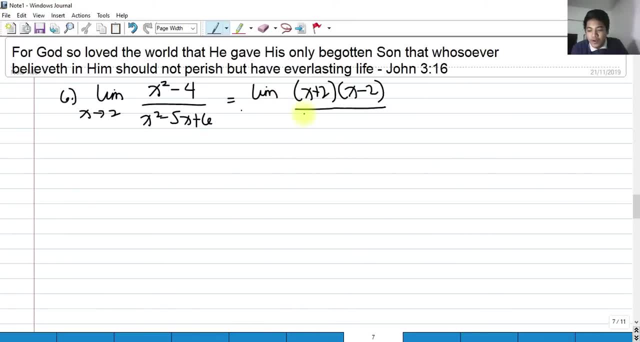 squared minus 5x plus 6 if we factor that out. okay, if we factor that, that is x minus 2 multiplied by x minus 3. okay, okay, that's correct as x approaches to 2, as you can see here. okay, x minus 2. x minus 2. 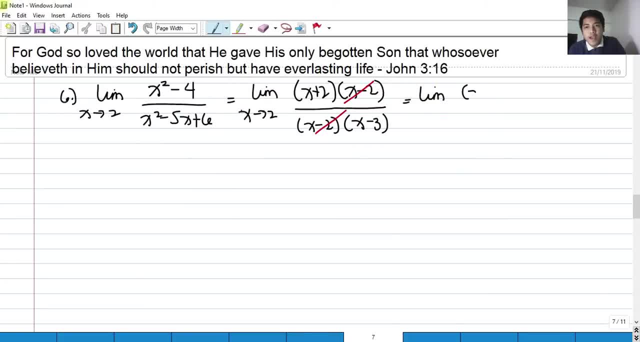 we are left with the limit of x plus 2 as x approaches to 2, over the limit of x minus 3 as x approaches to 2. so since these two are polynomials, so we can simply substitute the value of 2, 2 plus 2, and here we have 2 minus 3, so we have 4 over negative 1, which is negative 4. 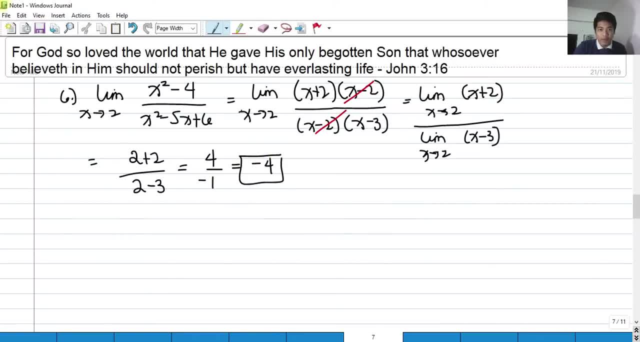 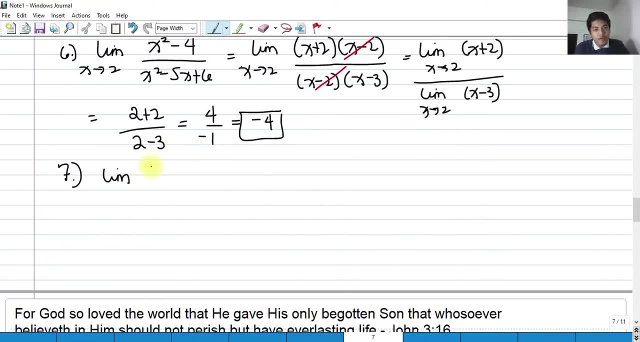 so that should be our answer for this problem. okay, and again, another problem, for that is that if we have the limit of x squared plus 3x plus 2 over x squared plus 4x plus 3, as x approaches negative 1, so the only thing that 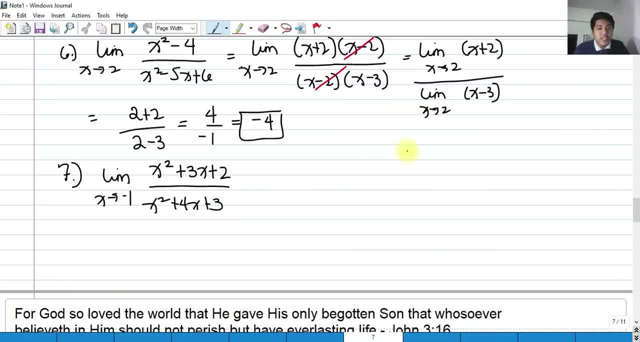 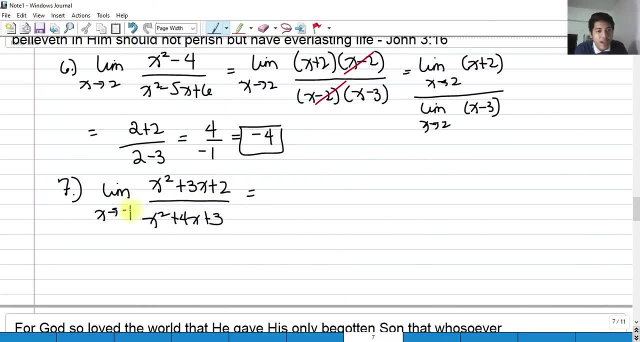 we are avoiding again is the denominator to get 0. but since this is a polynomial function, this is a polynomial function, we can simply substitute the value of a to our x's, so we have negative 1 squared plus 3 times negative 1 plus 2 over negative 1 squared, plus 4 times negative 1 plus 3. but you can also okay. 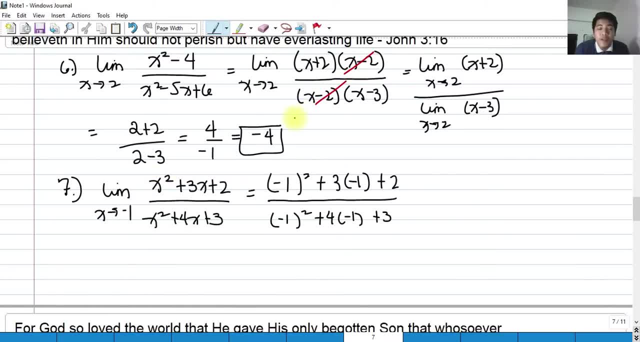 you can also factor this out, just like what we did on the previous example. if i'm going to solve this, number 6 directly substituting the 2, we will still get the same answer. okay, so i'm showing you the ways how to solve this, as long as the denominator should not be equal to 0. 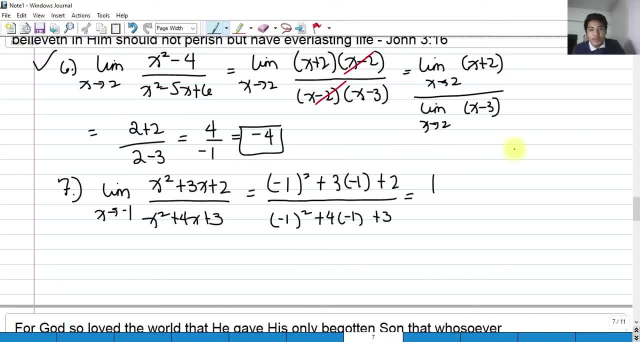 so negative 1 squared would be 1 plus 3 times negative 1, that's minus 3 plus 2. okay, over negative. okay, negative 1 squared is 1. so we have 1 minus 4 plus 3. so we have here: 1 minus 3 is negative, 2 plus 2. 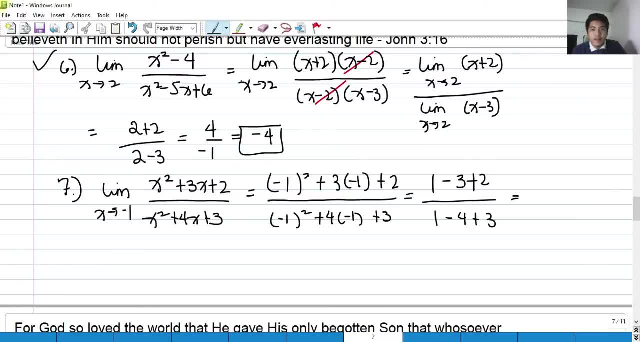 okay would be that would be 0 on the denominator and 1 minus 4 is negative. 3 plus 3. oh, we have an indeterminate form, so there must be a way to solve this. okay, so we cannot allow this to happen. okay, so that is not. 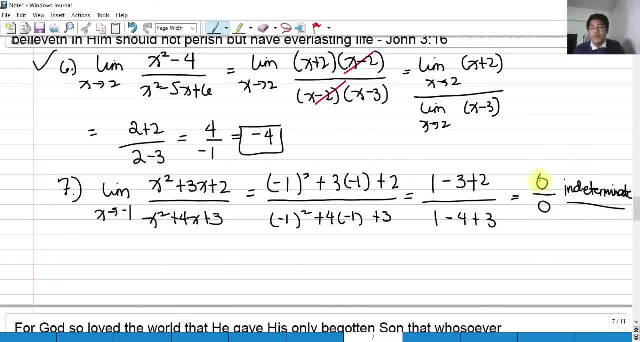 the answer. we have a denominator that is equal to 0.. okay, if the numerator is the only one that is 0, then it's fine. so it's an indeterminant. so what are we going to do? we're going to do, is we're going to? 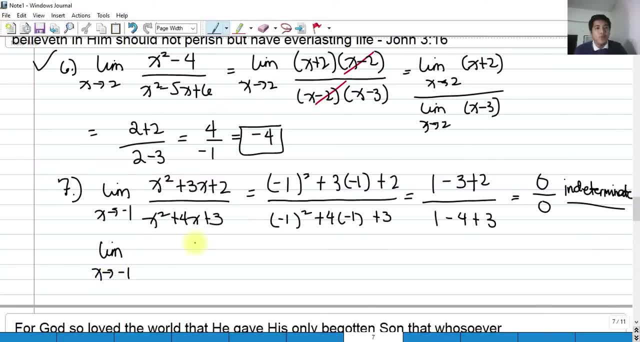 do is we should, what we should, factor or simplify this are just like what we did here. okay, so if this uh answer appears, that is indeterminant force, meaning that you will have to do something in this in our function. so if we simplify that x squared plus 3x plus 2 is simply x plus 1 times x plus 2. 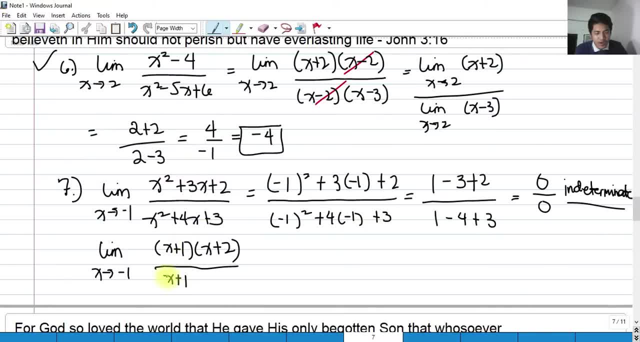 over this one is x plus 1, x plus 3, x plus 3, and x plus 1.. That is still the same. So, as you can see here, this x plus 1 would simply cancel. Okay, Leaving us we have the limit of x plus 2 as x approaches negative 1. 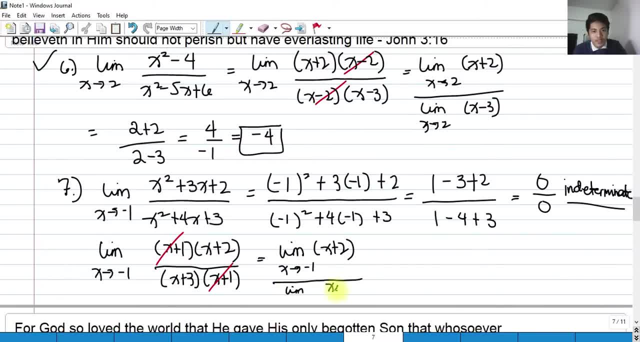 over the limit of x plus 3, okay, as x approaches negative 1.. So we have. we can simply substitute here, because this is a polynomial. So we have negative 1 plus 2 over. I'm doing the shortcuts okay. 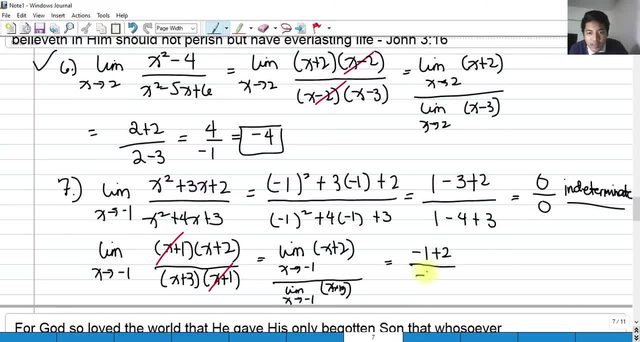 And we have limit of x plus 3 as x approaches negative 1. That's negative 1 plus 3. So we have 1 over 2. And our answer is 1 half Okay, So that should be our answer for evaluating this limit. 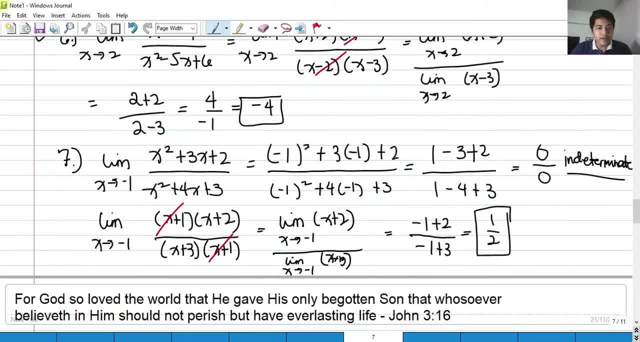 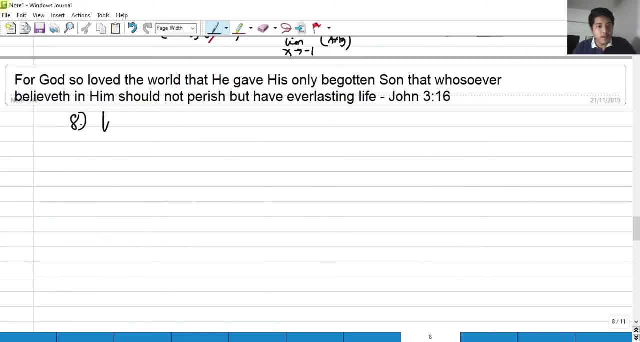 So down to our second, to the last problem here for our video. So we have number 8.. Okay, So we have to evaluate the limit of the square root of z minus 2 over square root of, I mean z minus 4.. 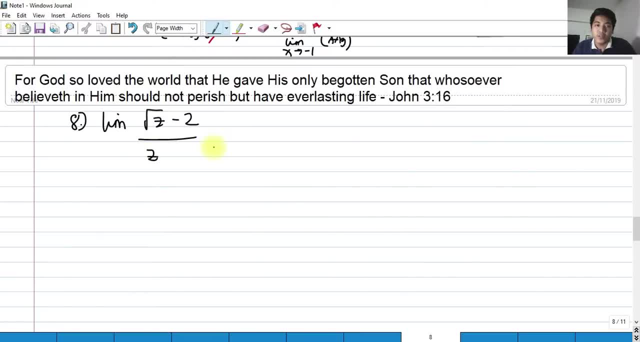 Okay, So the variable being evaluated, The function, is not always in terms of x. It can be some other terms. okay, other variables as z approaches 4.. Notice that if we substitute directly 4, okay, 4 minus 2, square root of 4 minus 2 is 4 minus 4.. 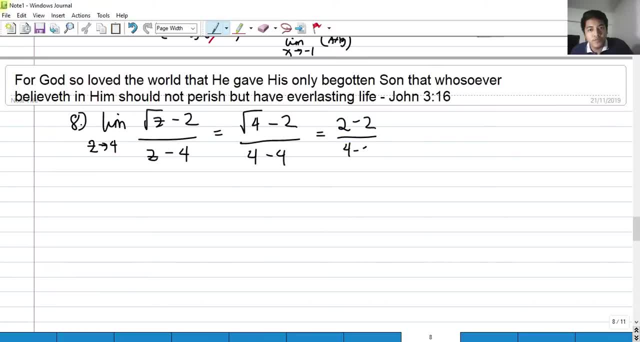 So square root of 4 is 2 minus 2, 4 minus 4.. So we would be having an indeterminate form that we cannot allow that. Okay, So we would be having an indeterminate form that we cannot allow that. 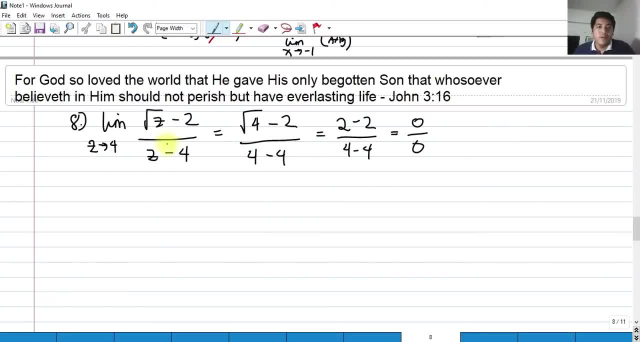 So we would be having an indeterminate form that we cannot allow that. So we must do something first. okay, in order for us, before we evaluate the limit. So what are we going to do is that we are going to multiply the function square root of z minus 2, okay, over z minus 4 in the conjugate. okay, multiplied by the conjugate of the numerator. 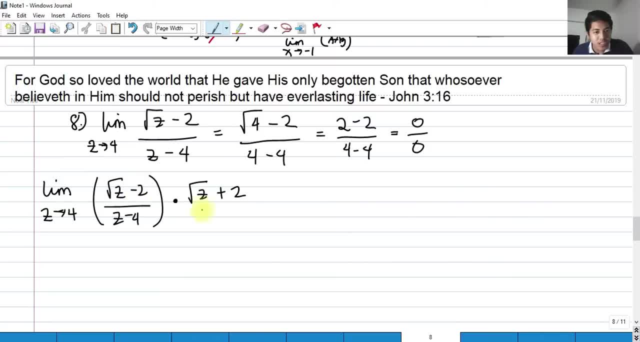 So square root of z. So square root of z plus 2, we would simply change the sign over: square root of z plus 2.. Technically, this is equal to 1.. Square root of z plus 2 over square root of z plus 2 is equal to 1.. 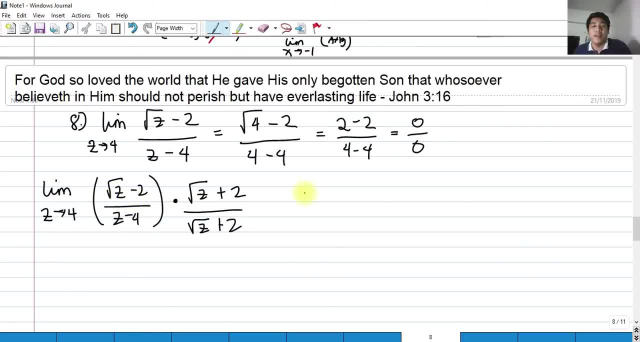 So multiplying it to our function would not do anything but would simplify actually our function. okay, This is still equal to 1. So it's still good to apply that. It's still valid to apply. to multiply that by this: 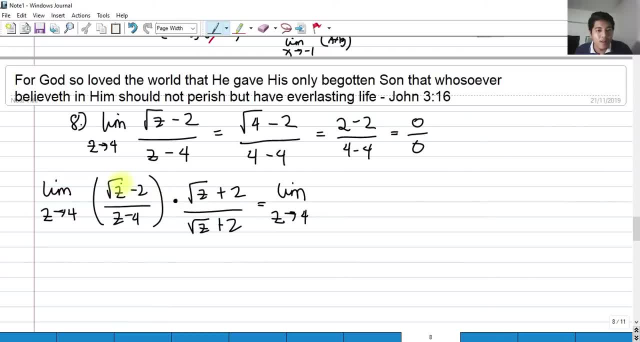 So if we multiply this, what will happen? Foil first, Square root of z times square root of z is simply z. Their exponents add up because we multiplied them Outer. that is plus 2 square root of z, 2 times the square root of z. that's the outer. 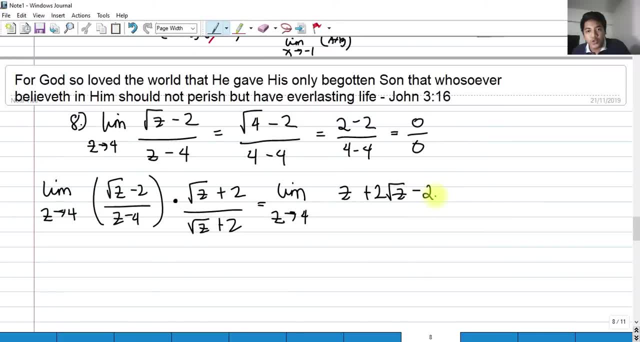 Inner negative 2 times square root of z. that should be minus 2 square root of z, Negative 2 and last negative 2 times 2 is negative 4.. As you can see here, 2 square root of z minus 2 square root of z would simply cancel okay. 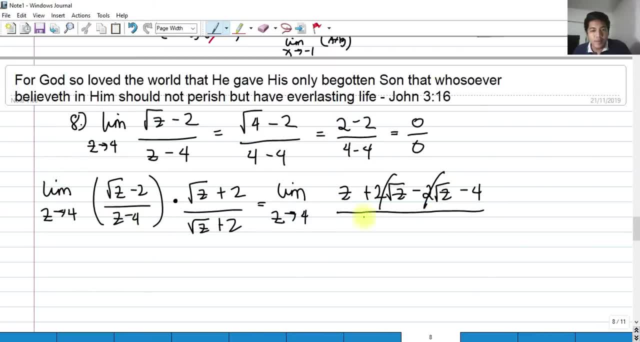 Okay, And we have on the denominator- let's not perform FOIL first on that Square root of z plus 2.. So we still have that. So we have the limit of z minus 4 over z minus 4 multiplied by square root of z plus 2.. 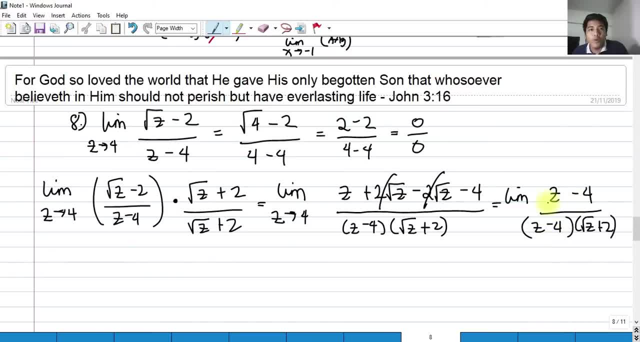 The reason I did not perform FOIL on that is because we can what We can- cancel this okay. So we have the limit of 1 over the square root of z, plus 2 as z approaches to 4.. So let's try to evaluate the limit. 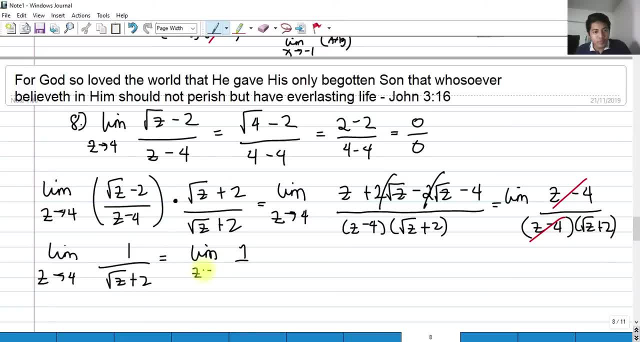 So the limit of 1 as z approaches 4 over the limit of square root of z, plus 2 as z approaches 4.. So the limit of a constant is the constant itself, So 1. So we have 1 over square root. 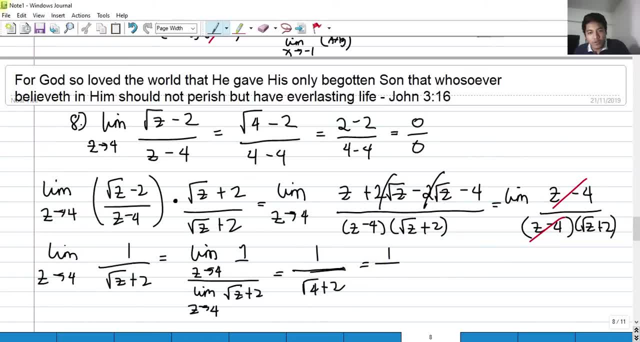 So we have 4 plus 2.. So we have 1 over square root of 4 is 2 plus 2.. We have 1 over 4, okay, So I'm going to leave you a problem. 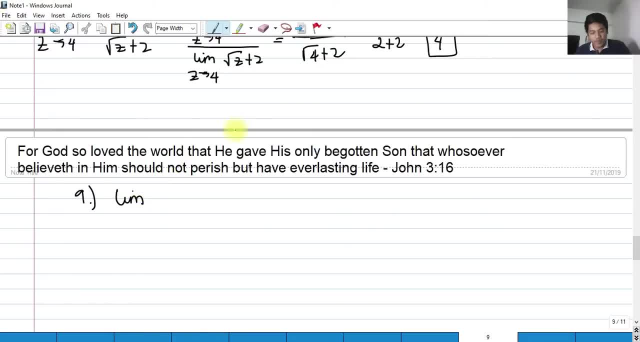 You can solve this on your own, okay. So the limit of the square root of 2x plus 22 minus 4, okay, Minus 4.. Minus 4 over x plus 3, as x approaches negative 3.. 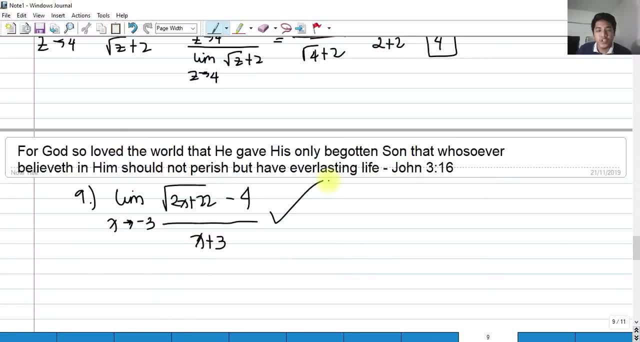 So this is your challenge, This is your practice problem. I'm going to leave you with that. Evaluate the limit of that And if you have already your answer, just comment down below on our comment section. And if you find this video helpful, don't forget to like or to comment down your comments. 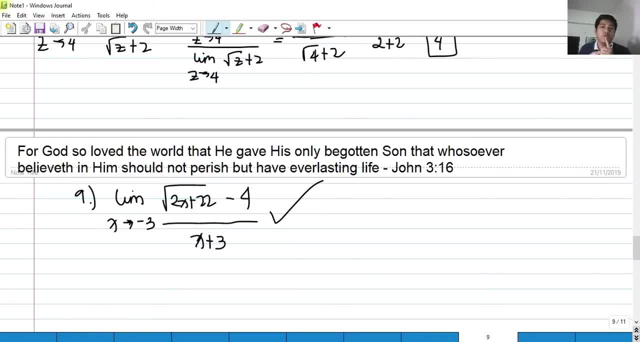 And don't forget, And most of all is to subscribe to my channel. So thank you so much. This is an introduction, all about the properties of limits and evaluating the limits. Again, this is Engineer Abad, and God bless you.